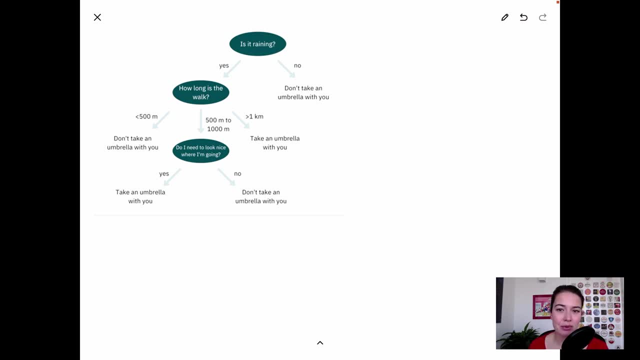 I'm going to the movies with my friends, maybe it's okay if I look a little bit wet. But if I'm going to a nice dinner with my- I don't know- girlfriends or boyfriends, parents, then maybe you want to look nicer, If you're like doing makeup or doing your hair, for example. So of 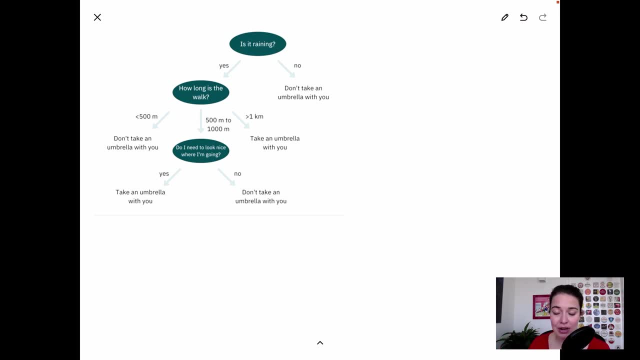 course. how does this happen? We create this tree based on a data right. So let's say we have a set of data. One column could be is it raining? Another column could be the length of walk. Another column could be the event index. I mean, I'm thinking of it as like: how nice do you need to look index Like if? 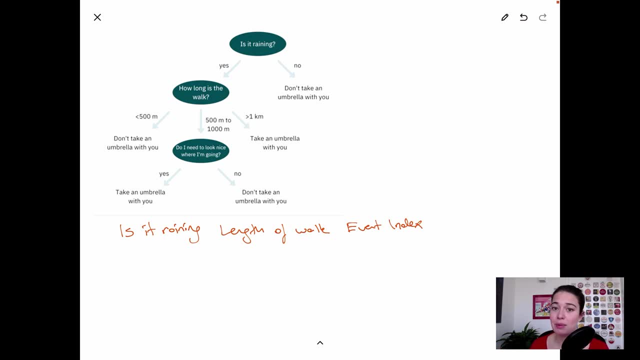 it's zero, then you don't need to look nice at all. If it's 10, it's definitely a place where you need to look super nice, let's say, And umbrella decision. Let's say: this is my kind of like data set And you know, it could be that. So you're basically basing this decision. 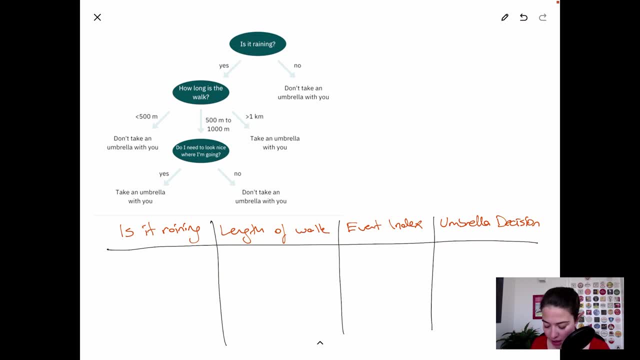 on your previous experiences. So let's say there was one time that it was raining, you were only going to walk 200 meters and you didn't really need to look so nice, So then you didn't bring an umbrella. There was another point where it was again raining and you needed to walk 750 meters. 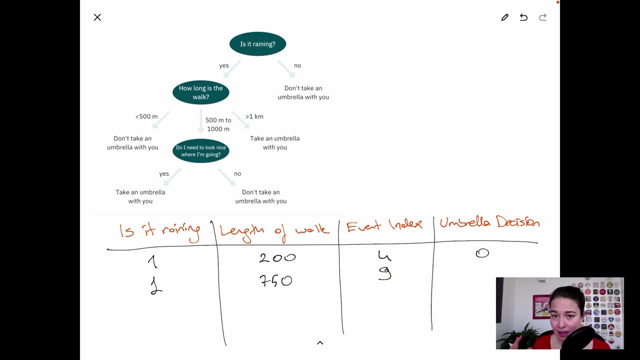 let's say, if it's like an event index of nine- I'm definitely making this up, by the way- And then you're going to bring an umbrella, And there was a time it wasn't raining, you only had to walk 500 meters- Let's make them meters- And it was kind of like an in-between event. And then you 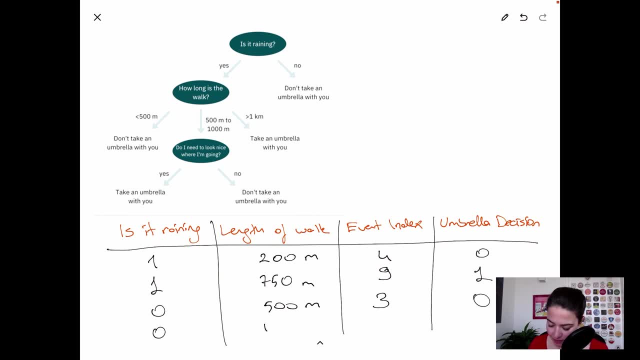 didn't bring an umbrella, obviously. And another event, let's say, where you had to walk like a thousand miles, a thousand meters, not a thousand miles, And it was like a nice-ish event, but you didn't bring an umbrella because it was raining. And then you didn't bring an umbrella because it 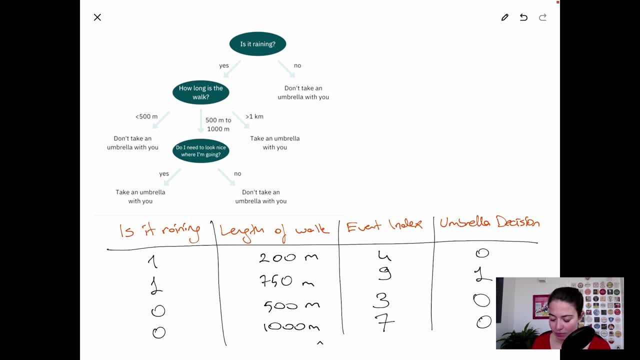 wasn't raining right, So that's an easy decision. So this is like one example of a data set that this tree might be based on, But of course, it's very simple. In this case it's very intuitive. But let's look into how these trees basically work. You can also call this a pseudocode. If you never 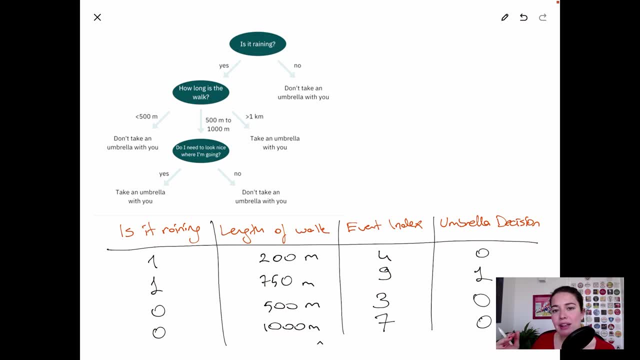 heard of this term before. it's basically like very high-level instructions of how the training will happen or how the tree will be created. In the case of decision trees. what happens is: you say so, you have all these columns right And this: 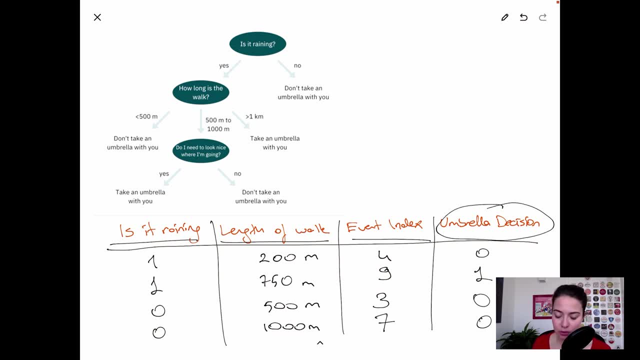 is a target column. This is what you're trying to decide. You might have more columns. of course, The trees are decision. trees are very good at deciding which one which columns to include or not, Because if a column does not is not contributing to the decision process, it will not. 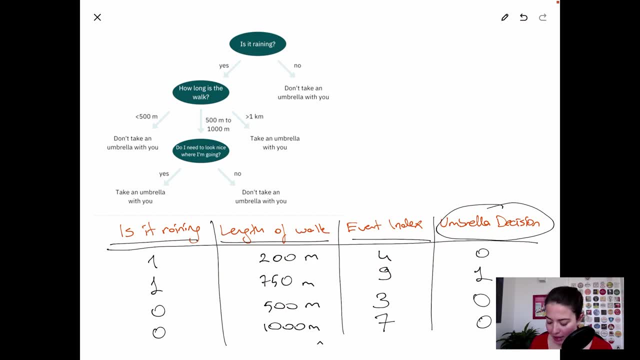 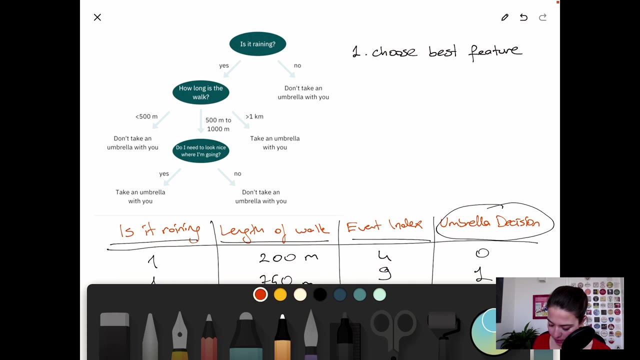 include it. So that's something important to know. Yes, So basically, what happens is, on the first step, the decision tree chooses the best column, or, let's say, feature, and it will make it. it will make it the beginning. 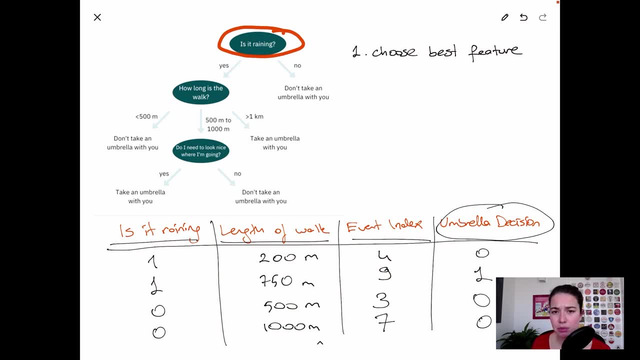 feature that we will be deciding. I think in some places this is also called the root. So that's the first thing that it does, And the second one it does is create the split Based on this feature. So, basically, what happens is here. it decided that it's going to go with, is it? 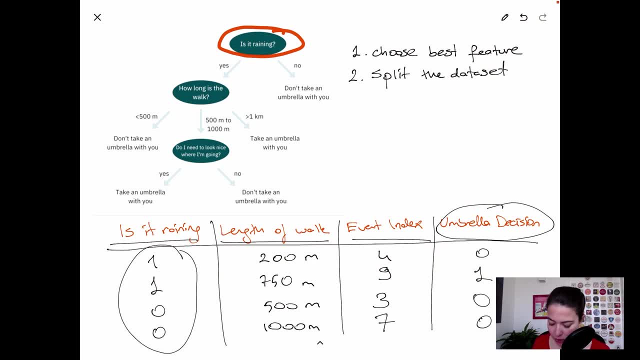 raining. right, And here it's this one. So then it says it's either is it raining, The answer is yes or the answer is no. So basically, what happens is it sends all the data points where the is it raining? 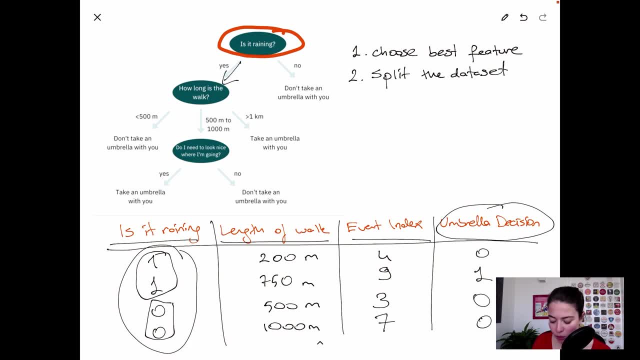 question is answered with the with a yes here, and all the ones that are not answered with a yes here. So, yeah, So, as you can see, when it's a no, it's going to say: is it raining, Is it raining, Is it? 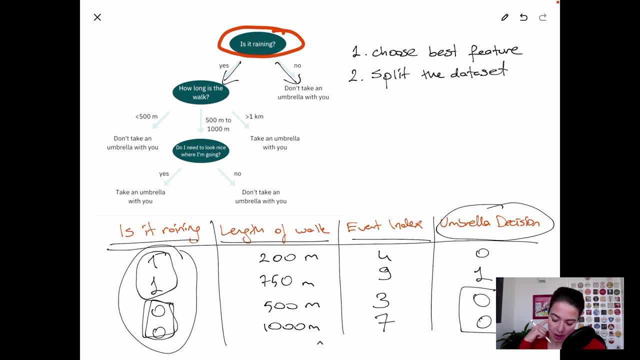 raining, It's definitely don't take an umbrella. And yeah, and these are the, these are the answers. And what happens is then it basically repeats it all the time, choosing the best one and the best one and the best one, one after another, And the last one is okay. how do we stop It? basically? 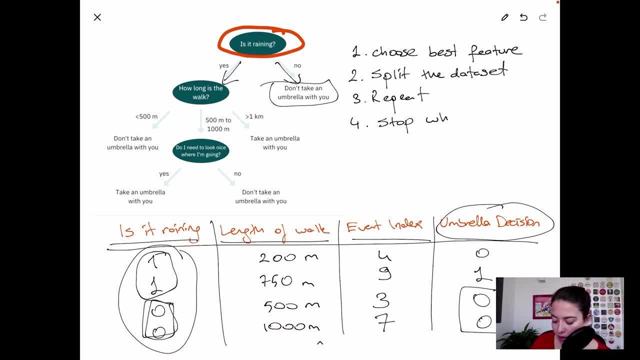 stops when the leaf nodes are pure. Okay, so I'm pretty sure already a bunch of questions popped up for you, So let's answer them one by one. Okay, what does it mean? the leaf node? The leaf node are the nodes that are all the way. 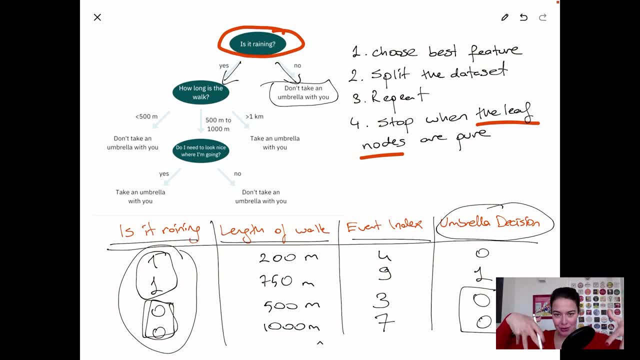 at the end. So I mean, of course, this decision tree looks like it's going down, But if you think of it as like a tree where the root is here and these are the leaves, So like turn it upside down, 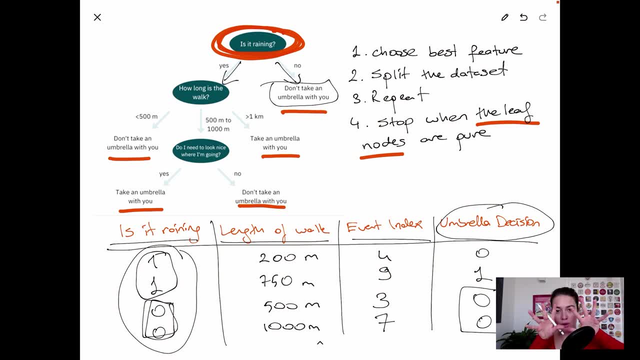 basically, These are the. these are what are called leaf nodes. So, like you know, all the branches go up and then at the end you have leaf nodes. So you know, all the branches go up and then at the end you have leaf nodes. 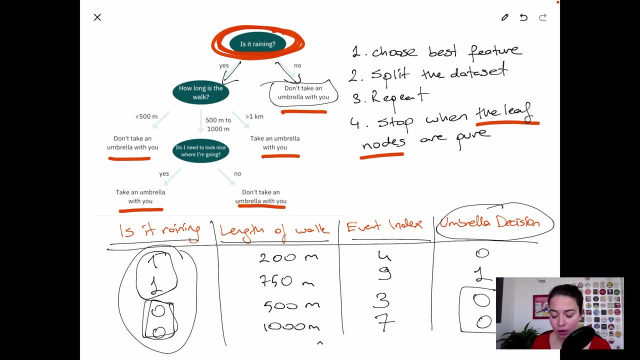 leaves A leaf node. being pure means that you only have one value. So it's here. we're working with zero or one right. So it's like, for example, this one: it divides it from yes or no, And like: 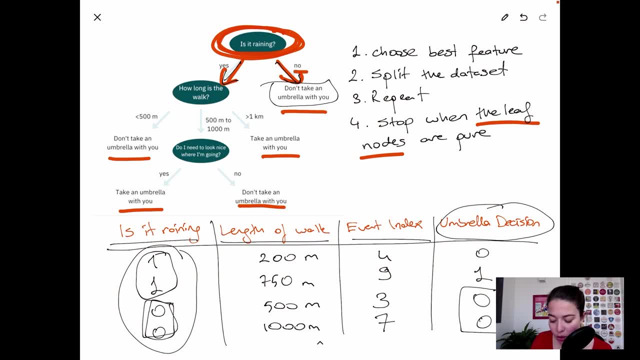 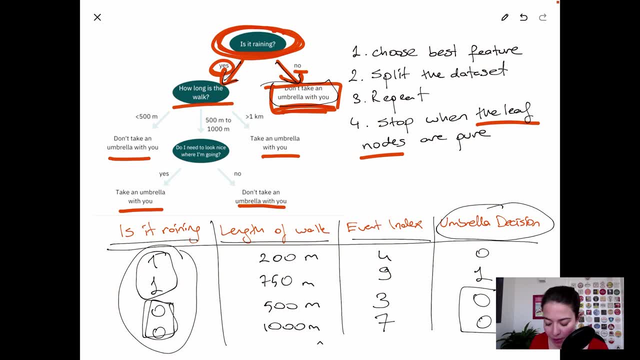 What happens is you still have some options, the possibility of it being yes or no. So it's not pure yet you have to divide it further to get pure nodes. So this is, this is a good thing to know. These are some just like general three terminologies, But of course there are some. 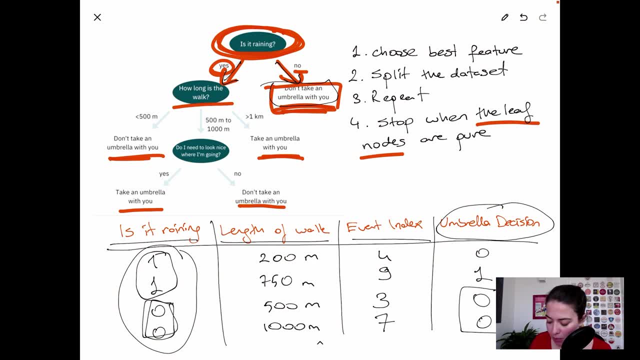 other questions that we want to ask at this point. So, for example, let me mark it with other colors. What does it mean to be the best feature? How does it decide that something is the best feature? What happens when this split needs to happen with a continuous variable? So here: 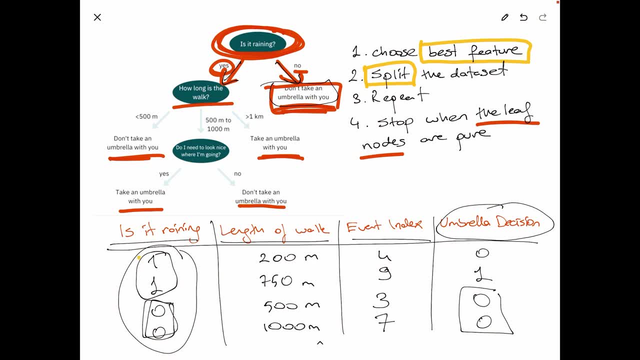 we've only seen. for example, the first one that we've seen is either zero or one right. What happens when it's a continuous variable like this? because this can be any value, this doesn't have to be 200,, 500, 1000, it can be 758, right. So how does it decide these values- 500,. 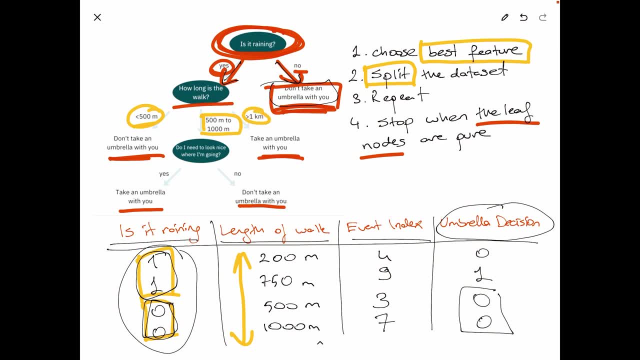 1000, or one kilometer. So that's the second question, This is the first, this is the second, not the best clarity. And the last question is also: how does it do the split when there is more than one categorical value? So you know, I could. this could be an example. the event index could. 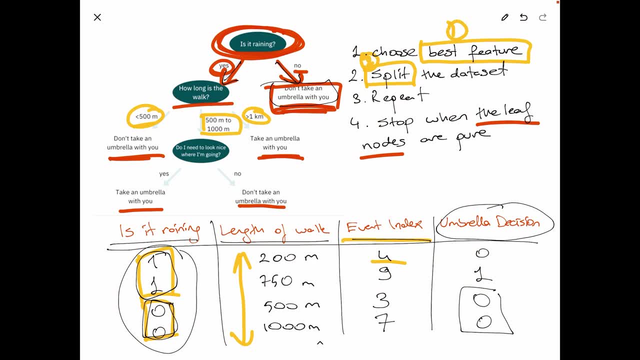 be an example for this. I mean, we don't really see it in the tree here. we kind of think of it as, like you know, this variable has been divided into either yes or no. But you know, when you think about it then you don't only have zeros or ones, you have. if you think of this as 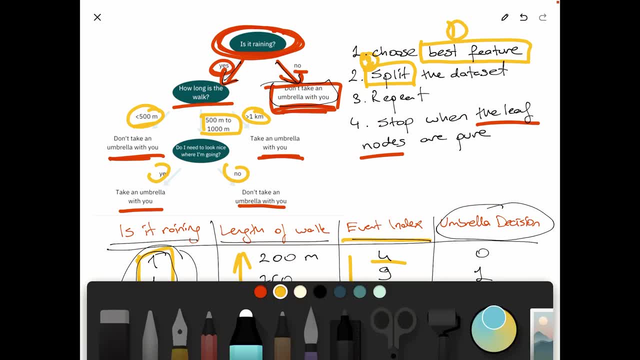 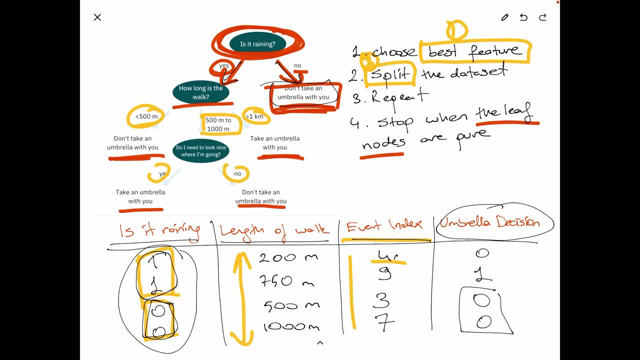 like categorical events. you know, you can also kind of like have it as, let's say, we can say: oops, this means dinner, This means I don't know, theater, going to the theater. This means chill with friends. 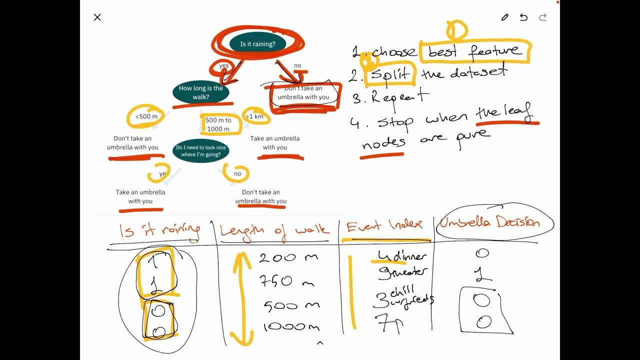 And this means picnic in the park. So, then, these are different categories that we need to consider, And how does it make the split when there is? how does the tree make the split when there are categorical and more than two categories involved? And, as a last question, we can ask: what is the difference between? 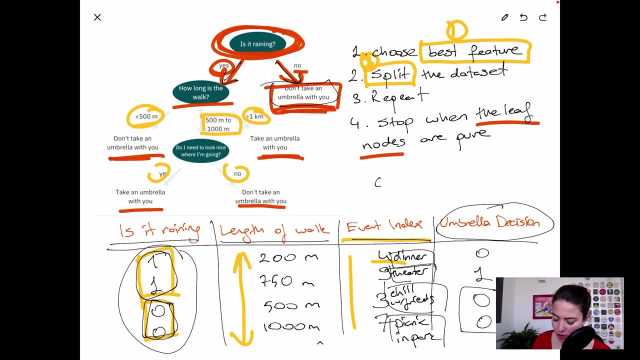 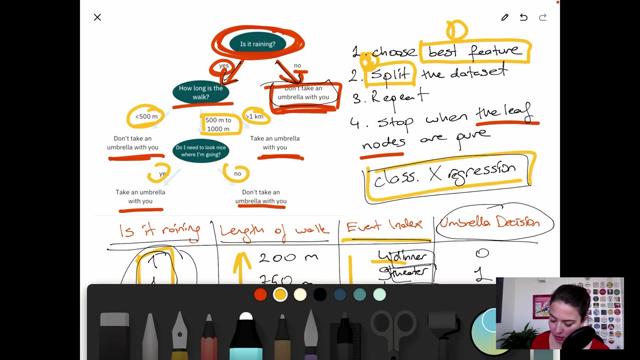 approaches of classification and regression. So what is the difference between classification and regression? So what is the difference between classification and regression And how do they happen? So this is yet another question that we want to answer. So let's start one by one and start answering these questions, All right? so let's start with our first question. 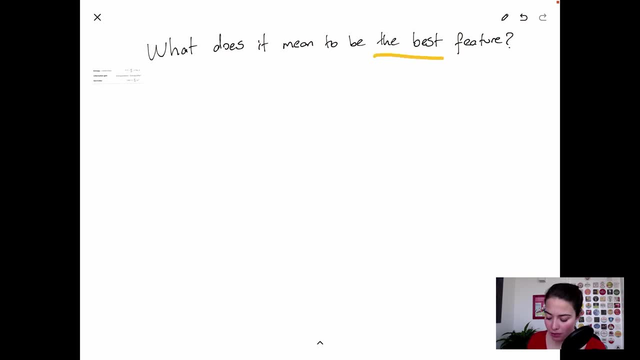 Our first question was: what does it mean to be the best feature? So, if you remember, I said that we divide, we make the splits in the data set based on which feature is the best, And this is basically where we come to a cross-reference. So, if you remember, I said that we divide, we make the splits in the data set based on which feature is the best, And this is basically where we come to a cross-reference. 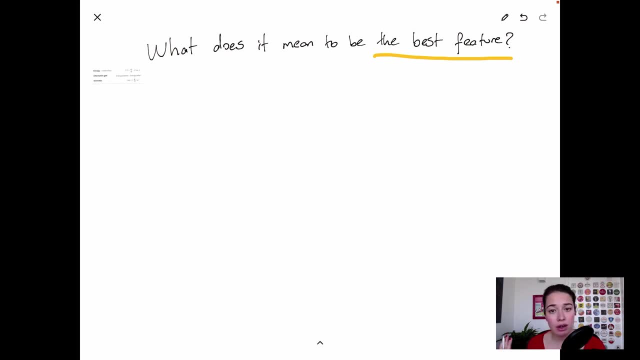 So, if you remember, I said that we divide, we make the splits in the data set based on which feature is the best, And this is basically where we come to a cross-reference. That's also a possibility, So let's just put a little star here to show that it's the default one. 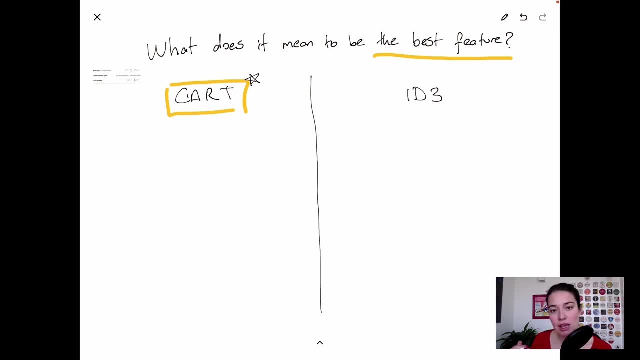 So how are they different? Basically, they are different in how they determine which feature is the best one. So the CART algorithm is using something called Gini index And the ID3 algorithm is using entropy. So I will not go into the details of how we calculate these things, But basically, entropy is a measure of 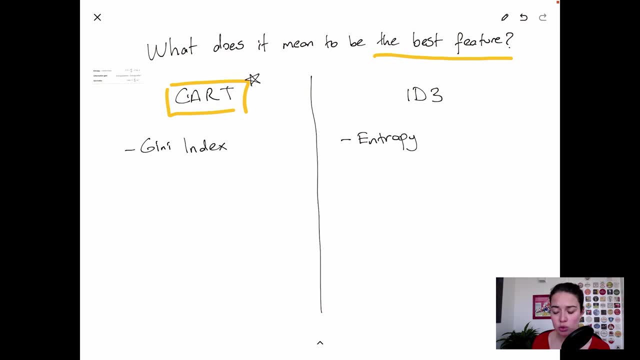 randomness, And it's a measure of randomness And it's a measure of randomness And it's a measure of randomness. If you ever take a chemistry course, maybe back in high school, you might remember it from chemistry. It's basically the same concept of how things are random. 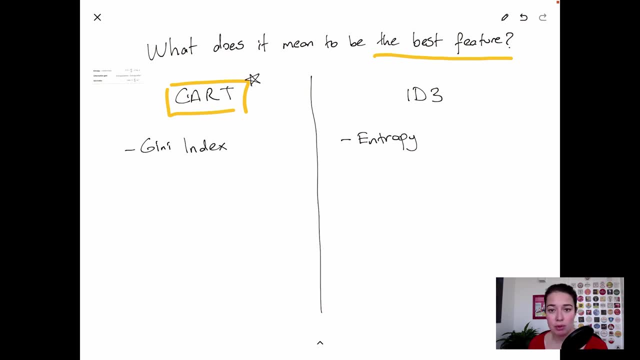 So let's say a coin toss, for example, I think is a very common example that's given Because the chances are 50-50 that it will either be 0 or 1, then the entropy is basically at its highest. It's, you know, cannot get any more random than this. 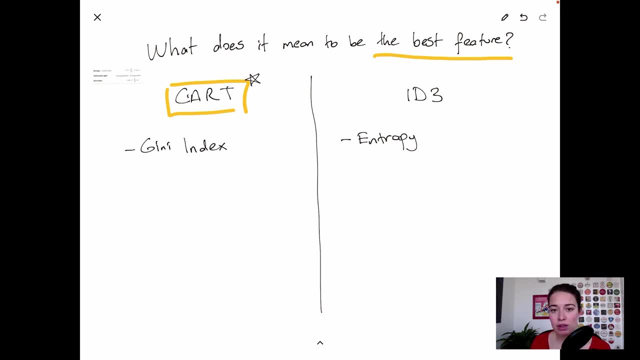 The more certain that you are that it's going to be one class or one outcome, one certain outcome, the more the entropy is lowered. basically For Gini index it's basically it's also called impurity- Let me also note that down. 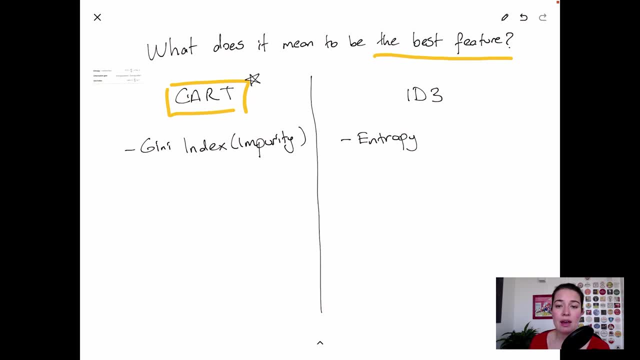 And Gini impurity is a measure of how pure the resulting nodes will be after the split. So if you manage to split a data set into two perfect sets, so let's say one branch or one leaf node is going to have only one class as a result. 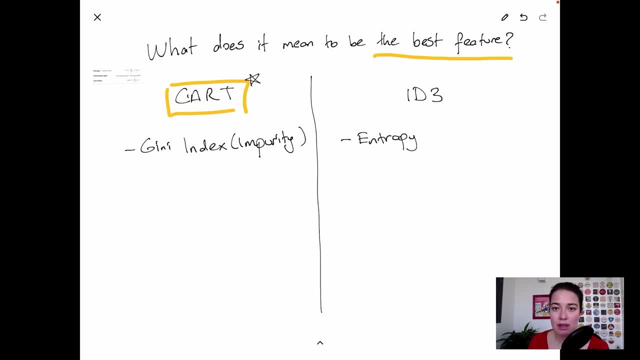 and the other one is going to have the other one, then you will be totally pure right. So that will be a totally pure result and that will give us a low Gini index. And on top of entropy we also calculate the information gain. 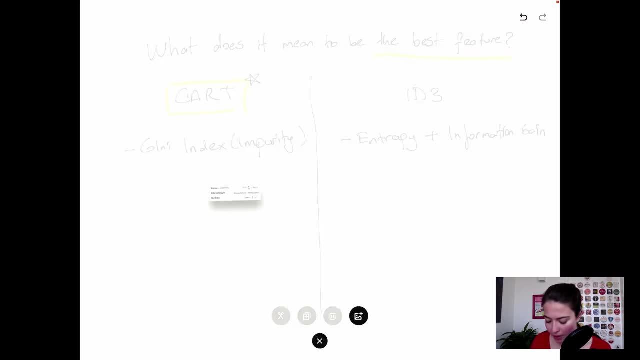 Let me just quickly show you how they are calculated, kind of like their formulas, But I don't think you should really like be scared of this, because it's actually pretty simple to calculate. I will also leave links to two of the articles that I found online which I think are very useful. 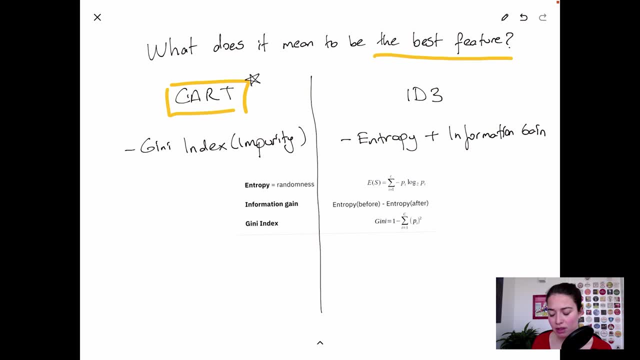 So I don't want to go through how this is all calculated and everything, but I think if you follow the examples there, you will have a really good understanding of how entropy and Gini index works. So basically, entropy, as I said, is just randomness and this is how it's calculated. 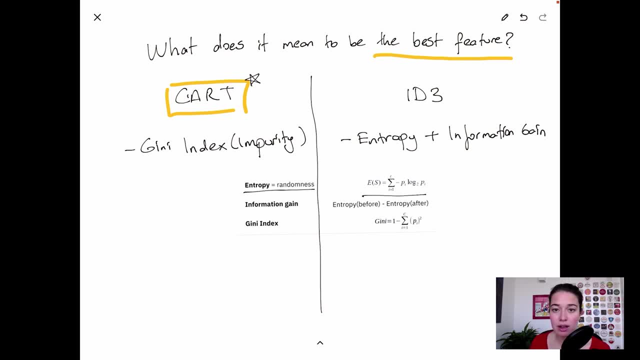 It's basically like the p's are the probabilities of each different category. same one for Gini index. it's again the probability of a certain category And information gain is calculated as what is the entropy before we do the split and what is the entropy after we do the split. 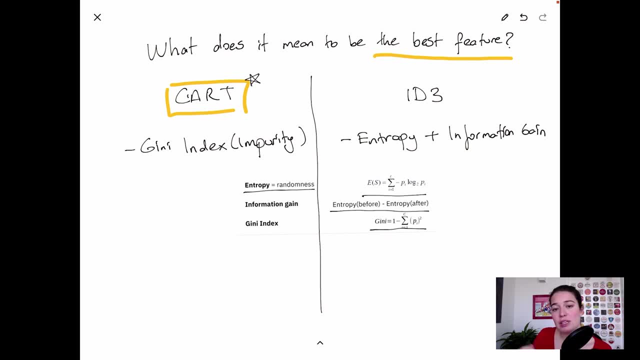 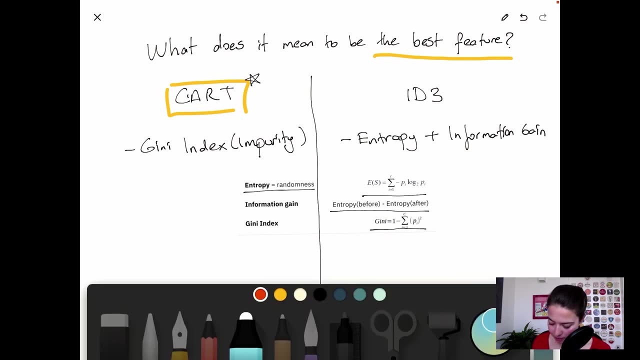 And for Gini index we mostly calculate just what's going to happen. what is the purity is going to be after the split. The main difference that you need to know here is the Gini index only separates things in a binary way, So 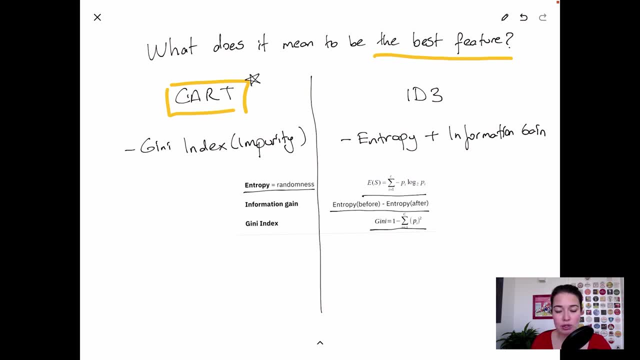 it cannot make trees that have nodes, that have branches, that have that are more than two. I think that was a very complicated way of saying it. so Gini index only creates branches like this. So it's either yes or no, but with entropy, with the ID tree algorithm, you can actually have more than two. 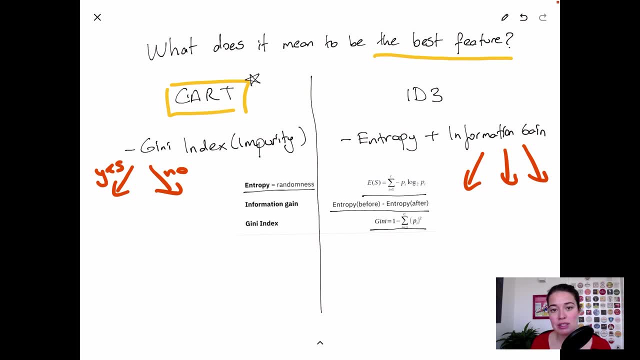 possibilities. So you know if you have some categories, let's say in your data set, it could be that you know category A goes here, B goes here, C goes here. You cannot do that with the Gini index. 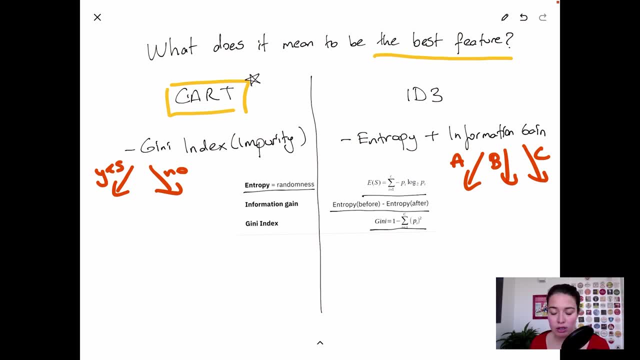 So that's the main difference. Not one of them is objectively better than the other one. There are upsides and downsides to using each, But yeah, we'll see more about how to implement this also in the next video, when I'm showing you how to implement. 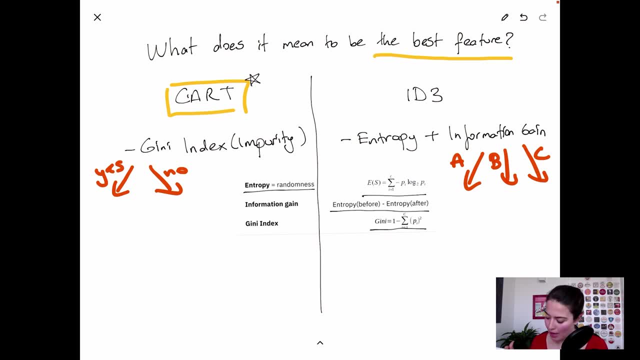 decision trees with scikit-learn and Python, But, as you might realize, these are basically greedy algorithms. So what happens here is, every time they look at all the features that are in the data, like the example that I showed in the previous page, and they look at all the features. 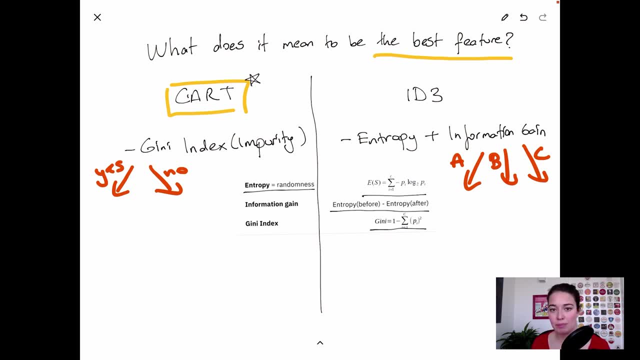 they calculate the Gini index and the entropy for both of the- sorry for all of the features or columns that we have for all the splits, and they decide which one has the best entropy or information gain or which one has the least impurity. right, So it is not thinking okay. 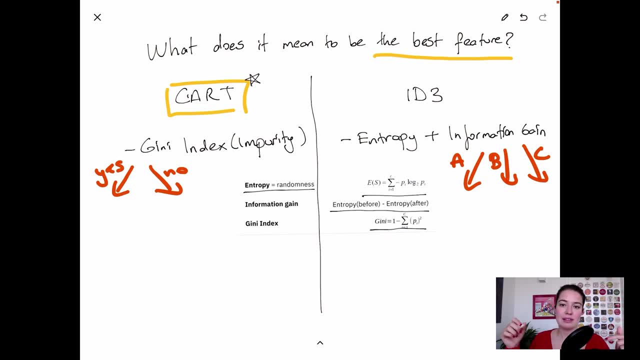 but what if I choose the other one, and then this one, and then the other one in the future? So maybe choosing a feature or column that has a lower information gain will help you in the future, But then that problem becomes very complicated. So that's why decision trees do not use this approach. 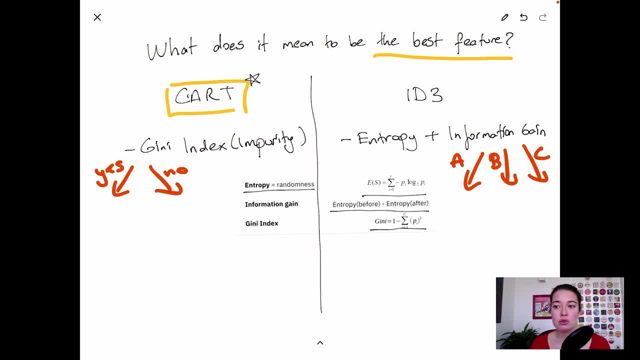 They just use greedy approaches Because if you try to think of all the possibilities of like choosing, let's say, column A and then column B and then column C, you're going to get into really complicated territory and the complexity of your algorithm is going to be very high. 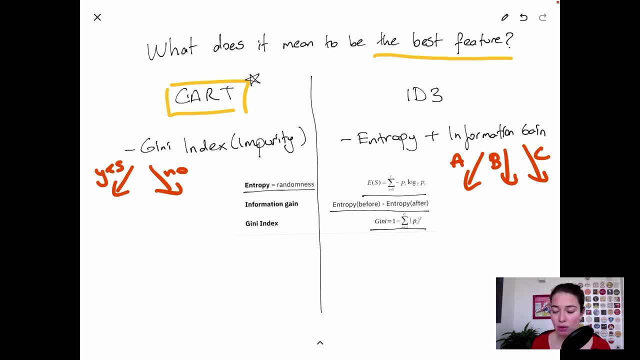 And it's going to take you a very long time to learn a very simple data set or fit a very simple data set. But with the greedy approach it actually creates maybe not the perfect tree, Maybe it doesn't find the global optimum, but at the end of the day it gives us a good enough. 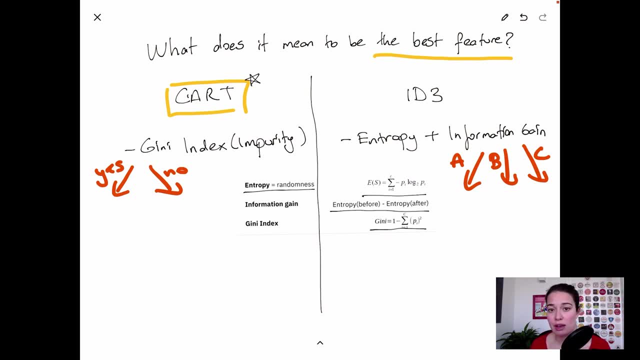 representation of the data set, that we will be overdoing pretty accurate predictions, let's say, on our data set. So that answers our first question: How do we choose the best one? Basically, we either calculate the entropy or the Gini index on all the features and we choose the one that gives us the least impurity, or 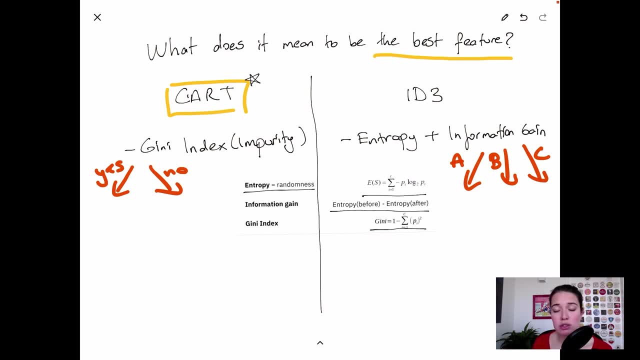 gives us the most information gain. And the next question that we had was how do we do this for categorical columns that have more than two categories? So, as you can see, for entropy we can have more than a binary split, So that's fine. 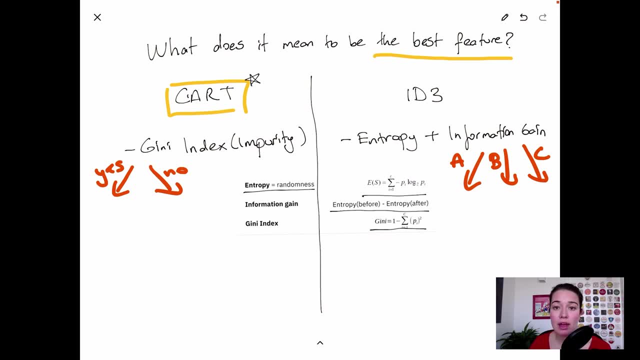 But let's say we have four or five values for a future. So I mean, you know if I need to show it as a data set, maybe this is feature one and we have a feature two, and then we have the target variable. right, 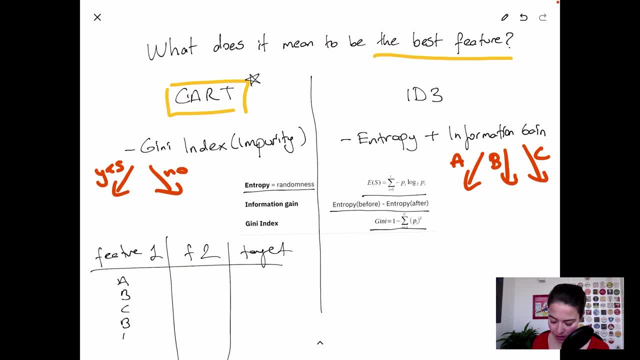 Let's say the feature one has like A, B, C, B A C. Let's say it can be anything. Feature two could be, you know, maybe it's like just zero or one, So and target variable can be anything. 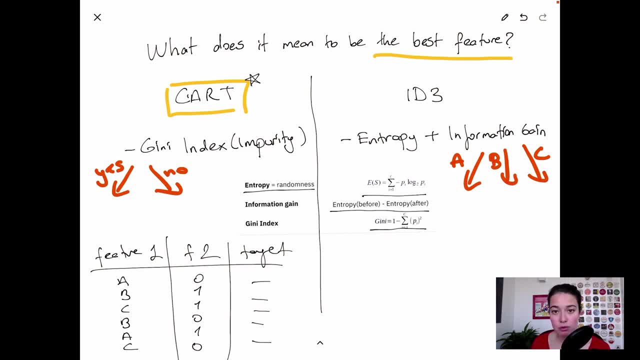 So how do we decide where to do the split for the Gini index? What happens is you can calculate the Gini index. You're going to have to calculate the Gini index for a feature one and feature two to see which one it will bring you a better purity. 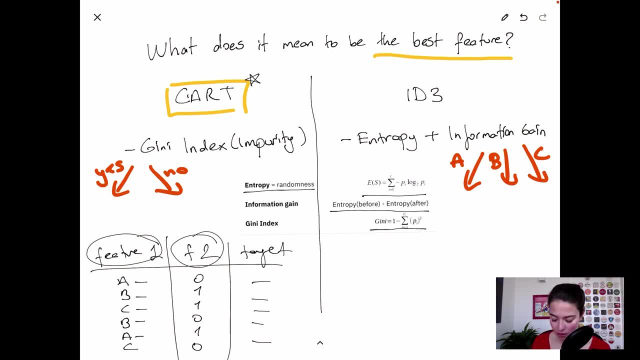 But you can also calculate it for each of these. So basically, you're just getting and seeing what will happen. if I separate it as is it A or not, Then this will go all the places where the data point has the future one value as A. So you'll be getting this one and 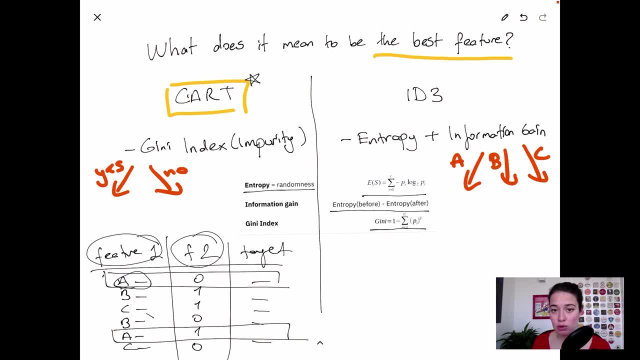 this one and then you'll look at your results. Okay, what is the Gini index for You just entered here like this and you're going to get that this is the future one. and what is this one going to bring you? a better purity? 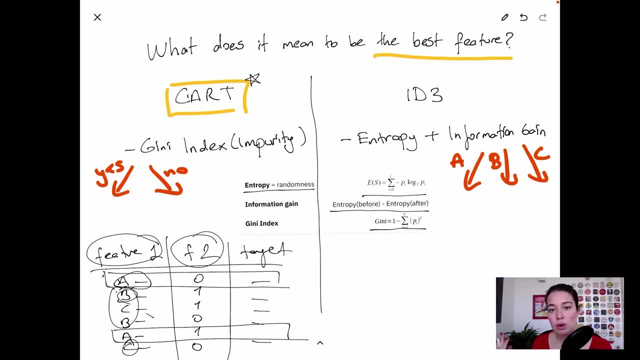 So it's like A against everything else and then you can calculate it for B against everything else and then C against everything else, And then see which one brings you a better purity or less impurity, and then select it that way basically. So that's how you do it. 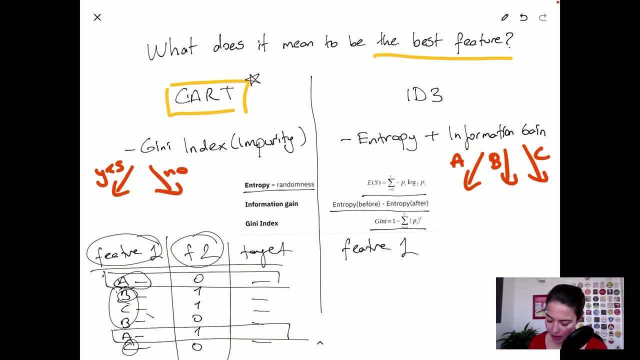 Another question that we had was: how does it work when you have a one and let's say, be the target variable, target variable, right, um, uh, we can say we have like two, four, six, uh, eight. let's see them as kind of sorted. let's say these are the values, uh, that we have. i 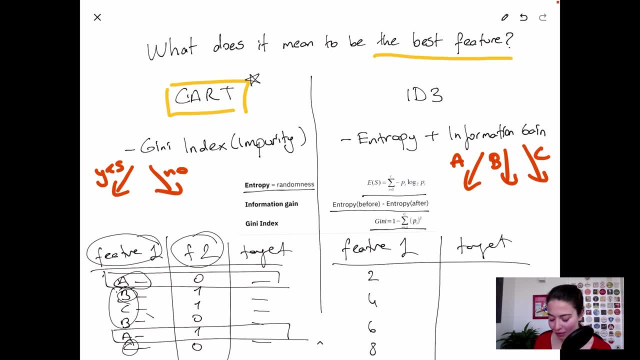 mean very easy for me mathematically, but what i learned is actually it's very neat. so these are the data points that we have, right, and when you want to find a point where you have to, when you want to divide it, uh, to make that decision, so say: you know, oh, if it's less than five, then go to this. 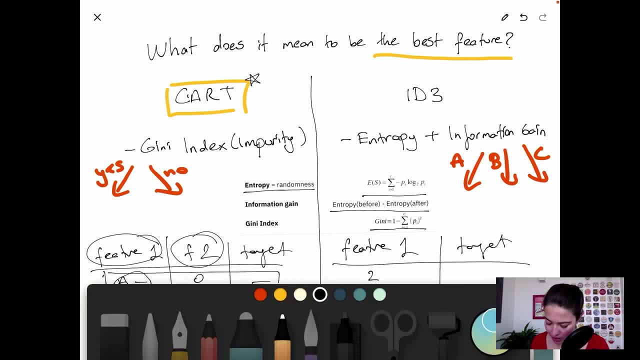 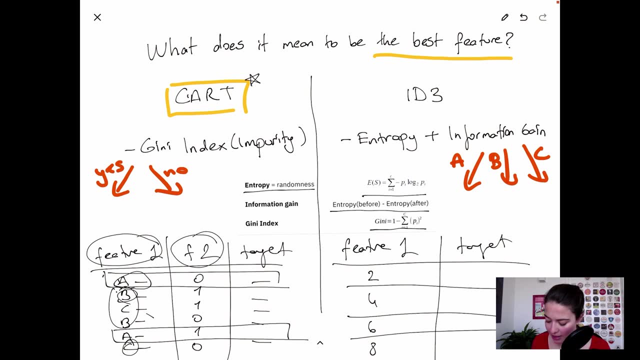 side if it's more than five go to this side. how do they do that? is they calculate the average of the values. so they say, let's say this is three, this is five and this is seven, right, and then you calculate the entropy or the genie index, thinking what happens if the future one is three and 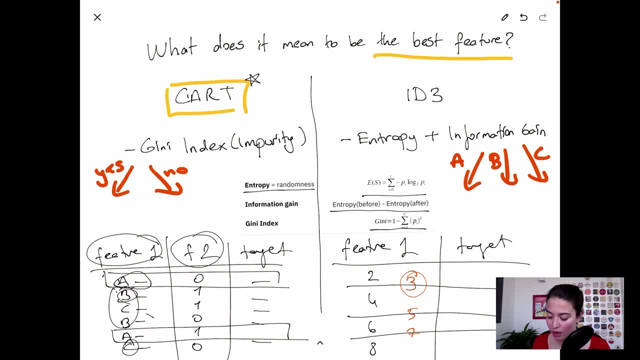 calculate the value of the future one, and then you calculate the value of the future one and then see and compare it to what you calculate when the future one was five or you know less than five or more than five, and do the same thing for seven. so you're basically creating some cutting points for 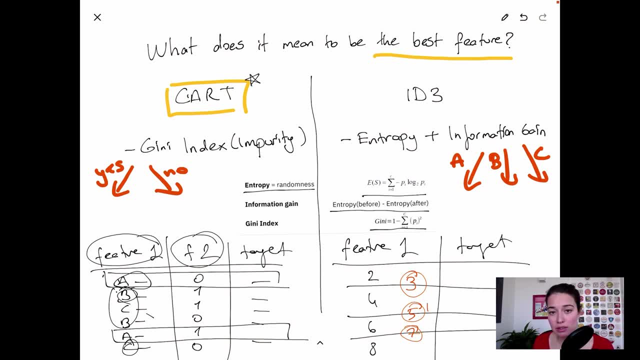 yourself and then choosing and trying to see which one will bring you more information, gain or more purity, and then you can decide and then say: okay, i want to see. i want to divide this as like: is it less than five? if it is less than five, go here. if it's more than five, go here. if it's more than. 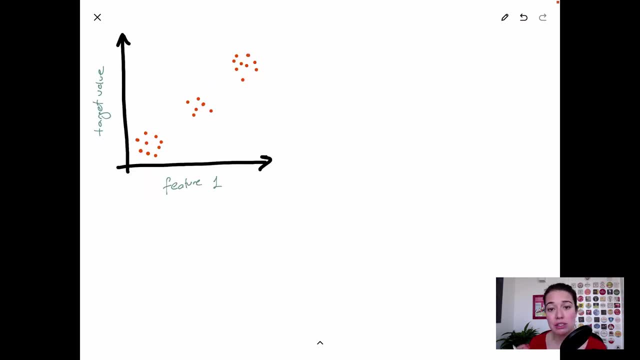 five. go here. everything we've seen so far was how the classification algorithm would work with decision trees, but we also want to do regression with decision trees, right? so here in the screen you're seeing a feature and how it corresponds to the target value. so if this feature is one, 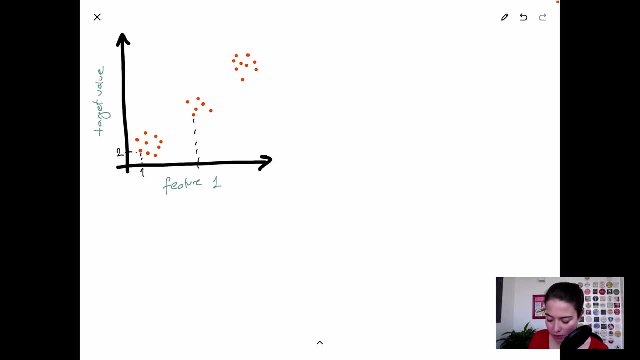 the target value, let's say, is two. if this feature is eight, the target value, let's say, is like 15, right, um? so the this is one way of showing how the feature corresponds to the target value. so you know what do we need to do? again, we need to choose the best feature. we need to choose the best feature to 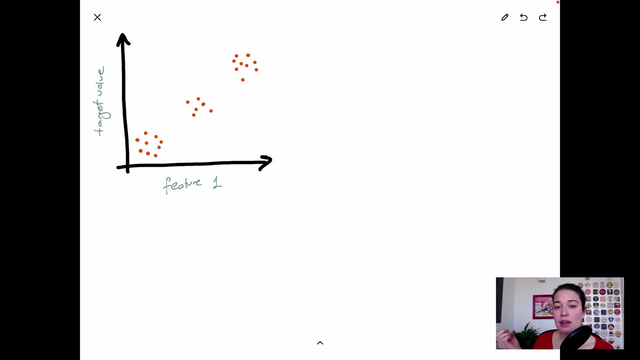 do the split and how do we do that? we compare the information gain normally of different features and here we're going to choose the feature that gives us the least error. but how are we going to do that and how do we know? do we have to separate it here? do we have to separate it here? do we have 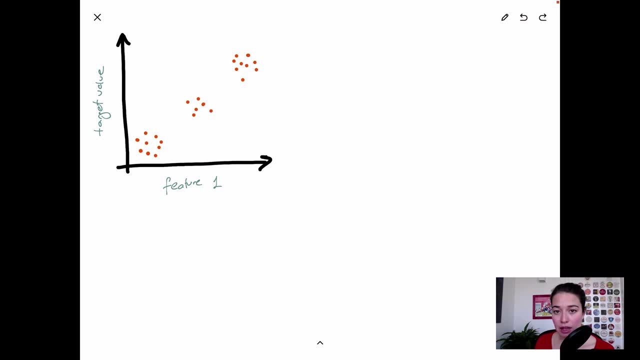 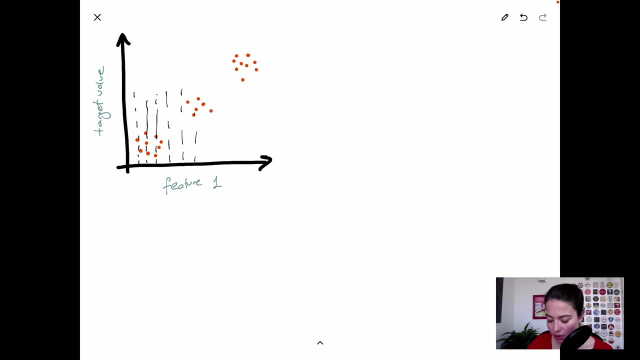 cutting points, possible or potential cutting points. it could be one, this could be one, this could be one, you know. so let's say these are all the possible cutting points, and then what you do is you compare these cutting points to each other. so let's say this is cutting point one, two, three, 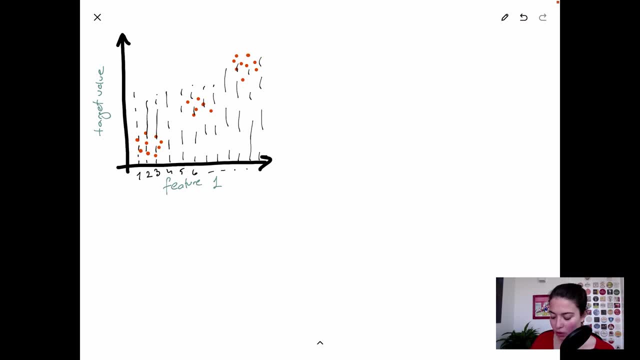 four, five, six, et cetera, et cetera. so then i will say: cutting point one, cutting point two, cutting point three, cutting point five, and then this goes on and on. then cutting point- uh, i don't know, let's say 15, all right, so what i do is for each of these points. 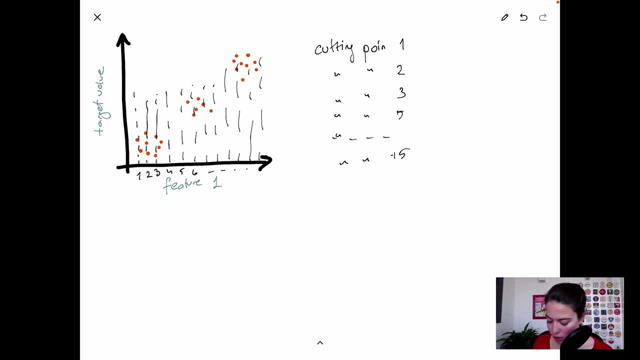 this can get a little bit confusing, so i'm going to try to go slow here. uh, i'll show you with the example of four. so this is one cutting point. right for each of these cutting points, i'm going to say everything that's lower than this cutting point where the future one equals to four is going to. 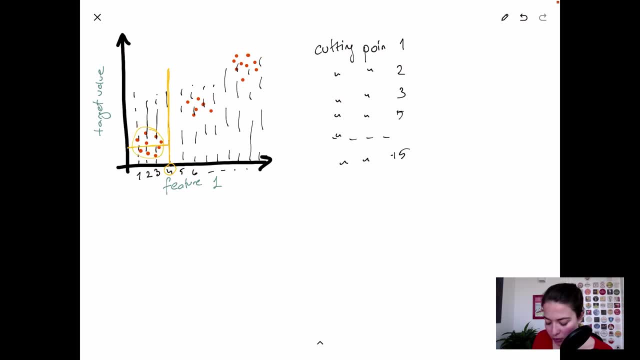 get the value of average of everything that's here. so average of these guys here, right? so let's say the value here is five. so i'm saying i'm going to make the. i'm saying one possible way of dividing is i'm going to say if future one is lower than, 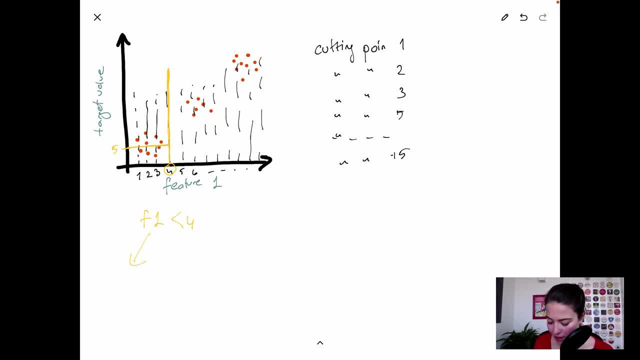 four, i'm going to make the division or the split uh, lower than four. yes, then the answer is five. if it's higher than four, i'm going to say: well, my prediction is, let's say, this corresponds to like 30.. so this is going to be 30. then i'm going to say, okay, then my prediction is: it's going to be 30.. 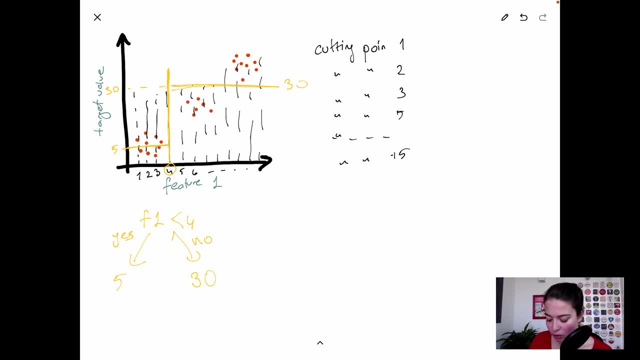 that's what i'm trying to say here. basically, if it's lower than four, my prediction is all of the average of all of these guys, and that is four. i saw that is five. and if it's higher than four, then my prediction is the average of all of these guys, which is, let's say, 30. all right, 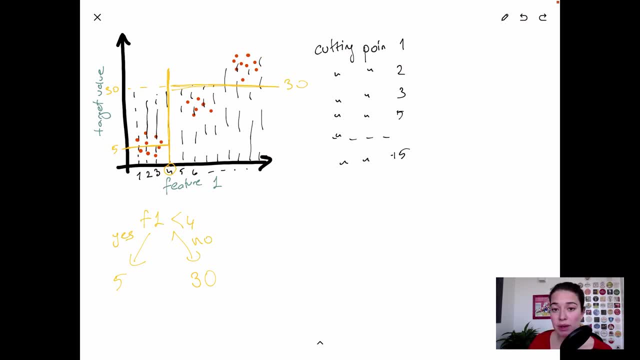 but how am i going to compare the cutting points to each other? so i'm saying this should be five, right then? i can basically, at this point, calculate the error that i get and how we calculate it is. we get the sum of squared errors and i'm looking at the error here, here, here, here, here, here, and 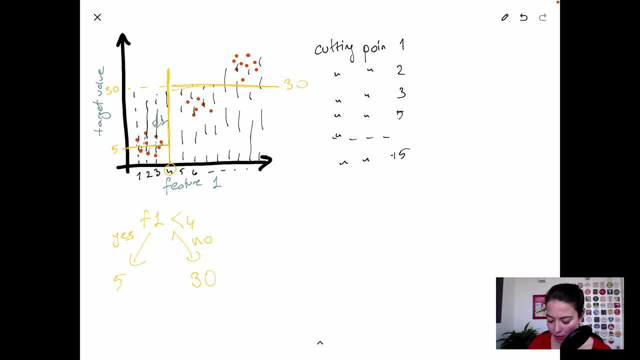 then i'm going to: this is going to amount to an error value, let's say one, or this is cutting point four, so let's say this is error four, and again i'm going to get the sum of squared errors here here, here, all of the error values. i'm going to get them and then basically, together, they're going to. 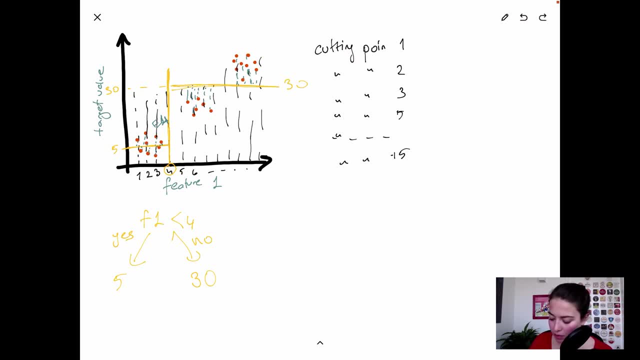 give me an error value, and then i'm going to get the sum of squared errors here, here, here, and then basically together they're going to give me an error value and then basically, together they're an error value and let's say, no, this is not it. uh, here error four right, and for each of them i'm: 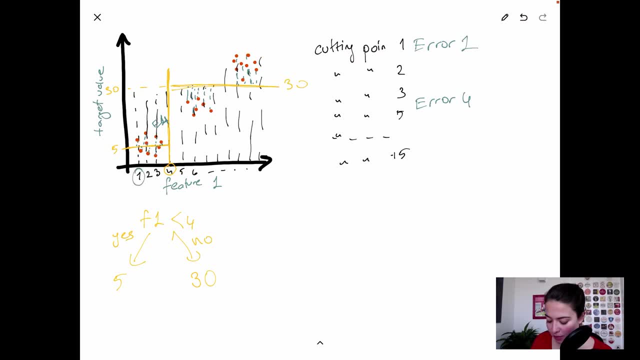 going to calculate the error, like, if i divided it at one, what will be the error? if i divided it at two? what would be the error if i divided it at three? what would the error? so on, so forth. um, so then let's give these like random numbers for now. 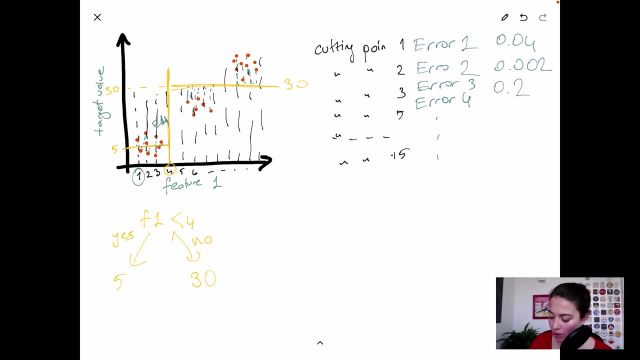 and okay, then i i calculate the error for thinking: if, what happens if i divide it here? what if it happens if i divide it here? what happens if i divide it here? and i am choosing the cutting point that gives me the lowest of all errors. so here it's this one right? so apparently, 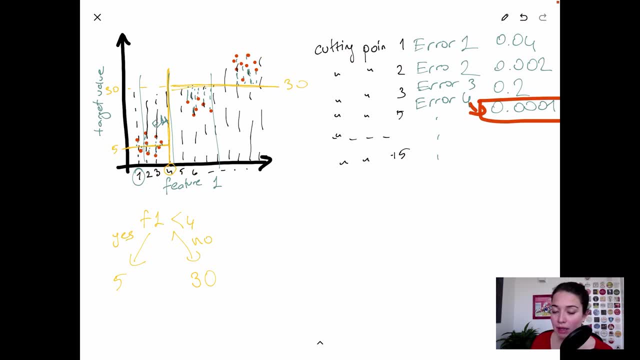 error. cutting point four is giving me the least error. so then i'm saying, basically going back one level higher, because we're doing this to compare features to each other, right? so if the data set looks like this: there's feature one, there's feature two, there's feature three and then the target variable. 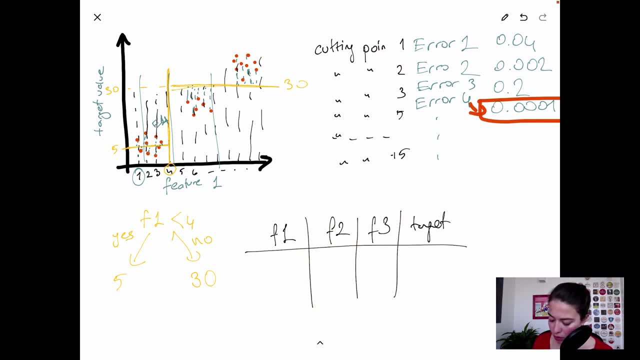 and i'm trying to choose which one to do the cut on and also where in the feature should i do the cut on. then i will say, okay, all right, let's say feature two is higher than four here, okay, and i'm going to say, oh, if i do the cut on here like this and that's the lowest. 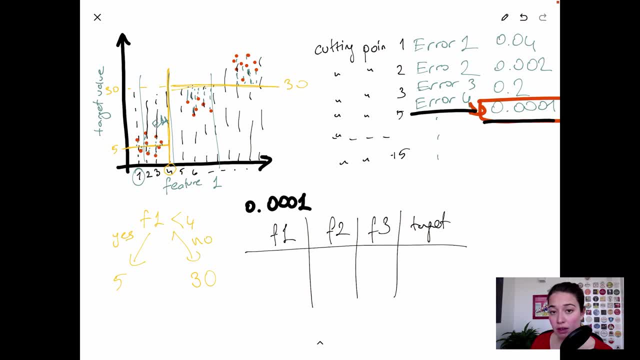 and then i'll cut on feature two and then i will say: okay for feature 1. error four is the lowest and it's this much okay. so if i cut on error 4, this will be the error. and then i'm going to do the same thing for error feature two. well, if i cut on feature 2, this will be the error. 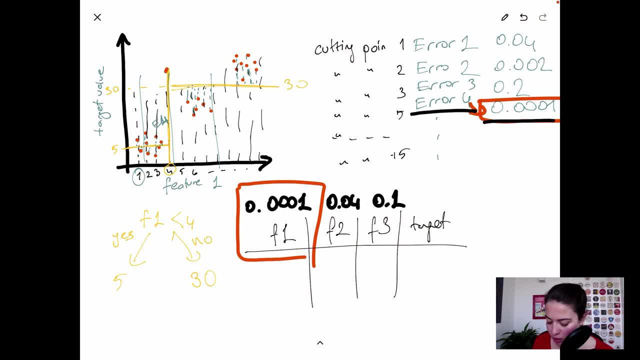 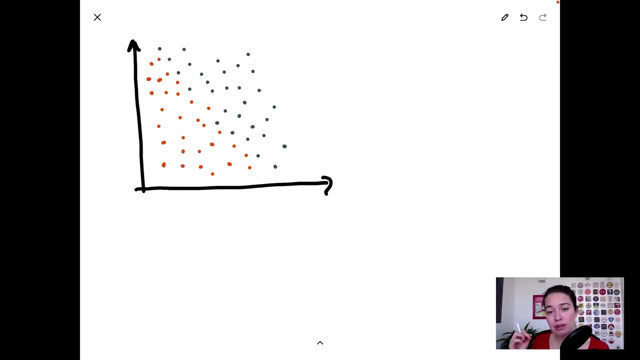 if i cut on feature 3, i look at all the possible options, going to say cutoff point 4 is the best option. So we learned how decision tree algorithms work, but there is one more really important thing that we need to understand about them, and that is that they tend to overfit. So if you haven't, 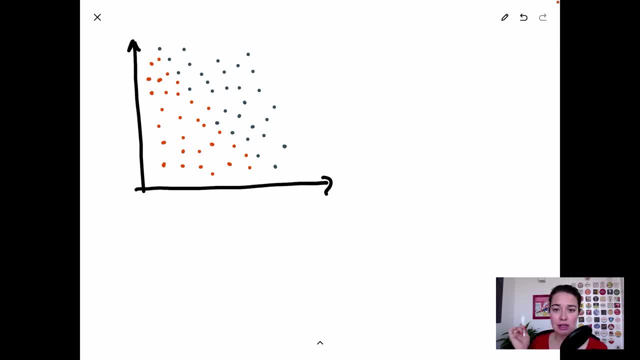 learned what overfitting is, and if you want to learn more about it, I will leave a link to my video where I explain what overfitting is. but generally, what happens is you know- let's look at this example data and how you would normally divide. it would be something like this, right? so yeah, maybe you are going to. 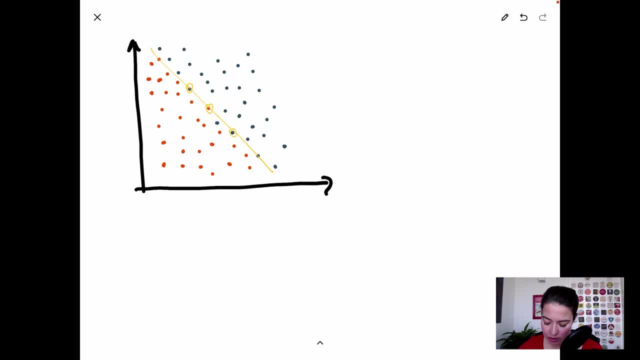 miss, predict this data point, this data point and these data points, but at the end of the day, your goal is to generalize based on the data set that you have. you're not trying to perfectly fit the data set, because the data set that you have is just some observations collected from the real world. it doesn't. 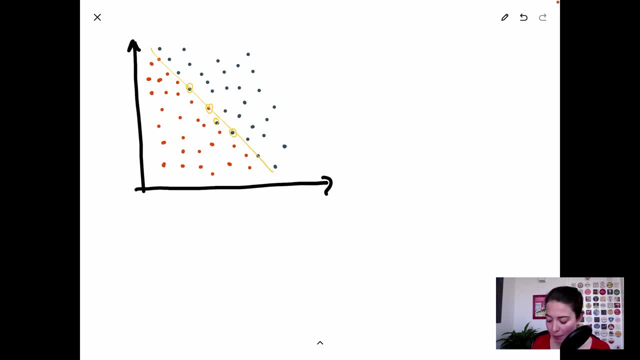 perfectly represent real world. but what happens when you overfit is that it will look something like this. so you're really trusting the data set that you have, basically, and you're saying, okay, this is a very rigid decision boundary, but this, this can cause a lot of problems and this is 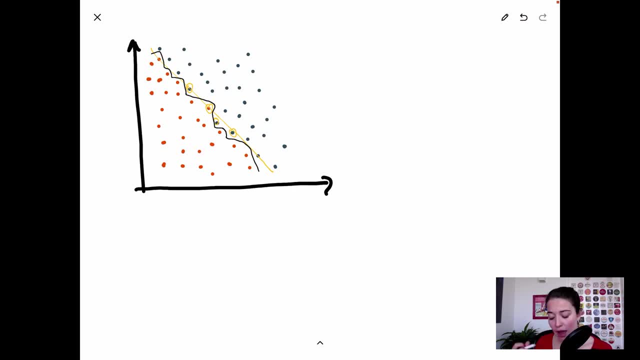 something that we don't want. we want to make sure that we're generalizing. how do we solve this with decision trees is one thing you can do is pruning. so this is pretty common to do. it's very common to do. it's pretty common to do. it's very 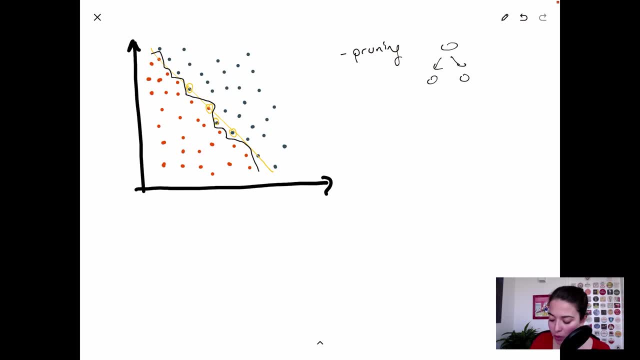 common to do. it's very common to do. it's very common to do it. if you're watching with real world, you can tell if it gets a lot numbers. so it's pretty common. so, basically, when your data, when your decision tree goes like this, you know it. 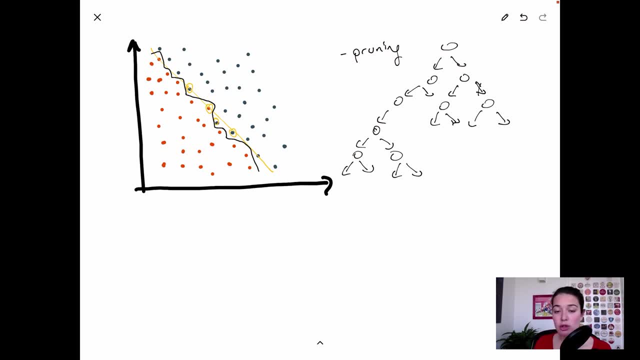 goes all around and then maybe like this, so it becomes like a gigantic decision tree, then what you can do is basically you are there algorithms to do this, but basically you're like looking at which say, okay, let's delete this one, this one and this one, and then basically make your tree a little. 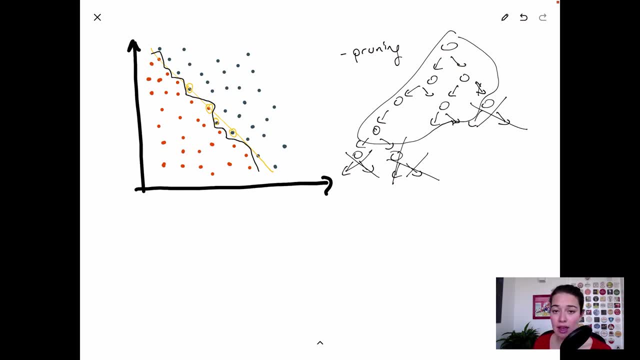 bit smaller it. it is not going to perfectly answer or predict all the data points or all the examples, but at the end of the day you're going to have a better machine learning model in your hands because it will not be overfitting your data set. another thing you can do is setting up. 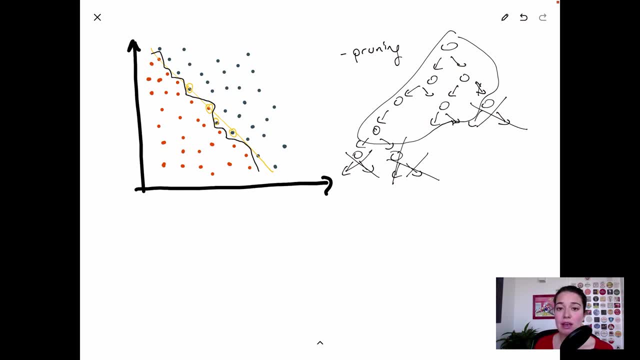 stopping criteria. so, as i said in the beginning, we normally- i mean normally- the algorithm is to run the decision tree algorithm until all the nodes, all the leaf nodes, become pure. so they are basically, they only have one type of data point in there. but instead what you can set is: you can 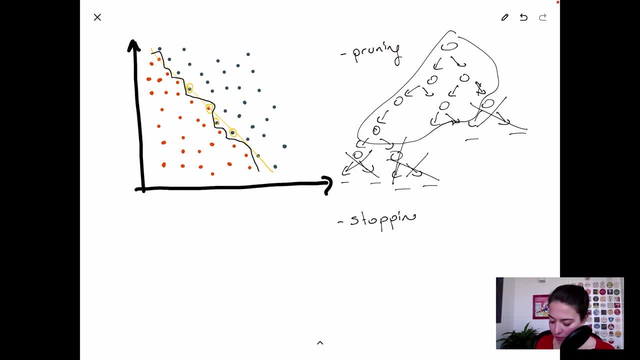 set some other stopping criteria. so let me and this stopping criteria. we will learn more about this in the next video. so thank you for watching and i'll see you in the next video detail when i'm looking or showing you how to do this in python and scikit-learn, but basically you. 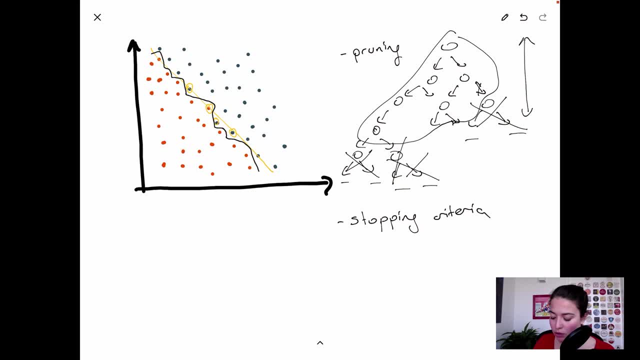 say the the depth of the tree, which is basically, like you know, that this is a zero step. this is the first, second and third and, as it goes like that, you can say: the depth of the tree can maximum before, for example. that's just one example. so these are some ways to stop the growth of the tree. 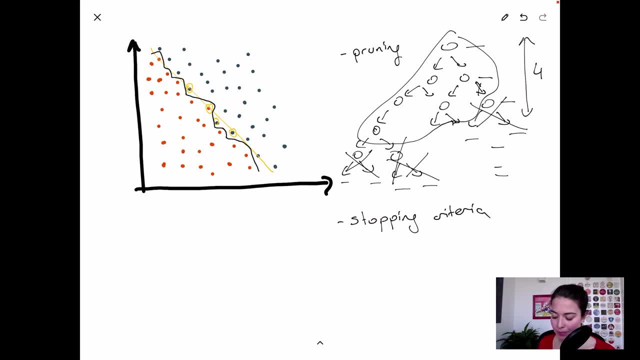 before all the leaf nodes become pure, and that way you can really stop or stop overfitting. and the last thing i'm going to show you is a little bit of a tutorial on how to stop the growth of. the last one is ensemble methods. so this is where, basically, you stop doing a decision tree, you know. 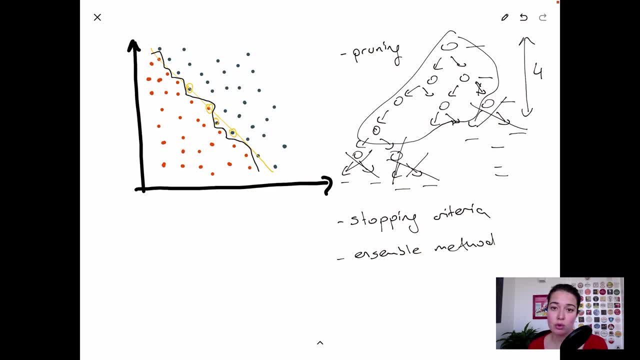 if you ever heard of it, there are. there's this other algorithm called random forests and with random forests you are bringing together a bunch of decision trees and in that way have them generalize better as an overall, better algorithm generally to do predictions on a complete in a 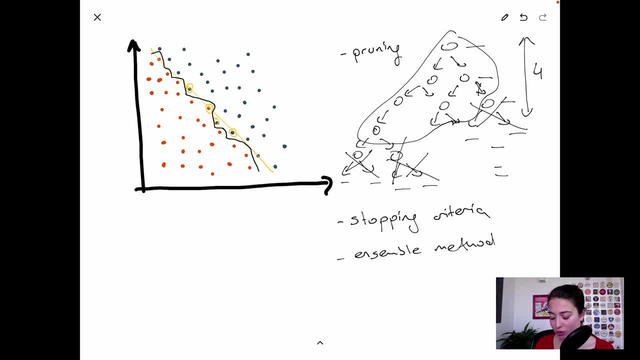 complex data set. so this is the last one, and i'll see you in the next video version, though this is the last option of how you can approach decision trees to kind of make them overfit less, um. but one last thing that i want to show you, also after overfitting, is: why would you? 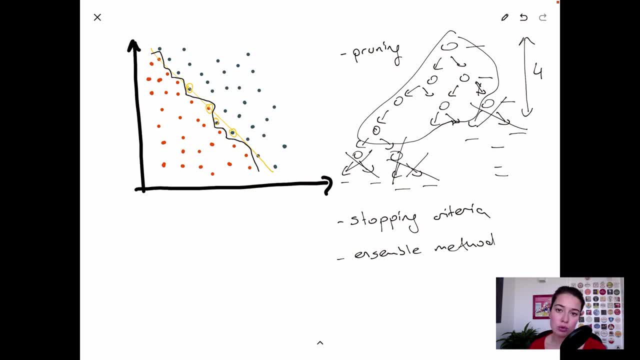 choose to work with decision trees, or why would you not? so the disadvantages of decision trees is. the first one is that they're very sensitive. um, if you change the data set that you're giving it, it's very likely that the tree is going to change, so you're not going to get the 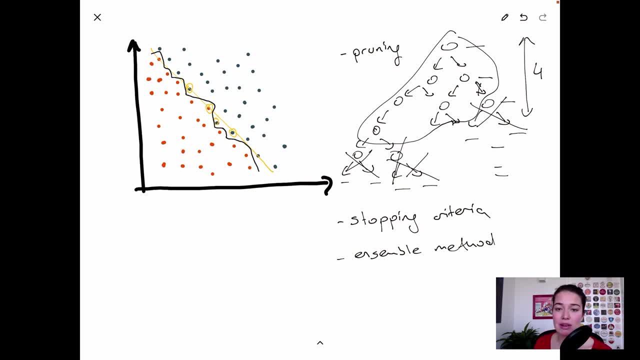 same tree every time you give it, uh, more or less even the same data set. so that's the problem. they're very sensitive and they're they very base the whole model on the data set that we, that they have. um, and generally the decision boundary tends to be very stiff and this kind